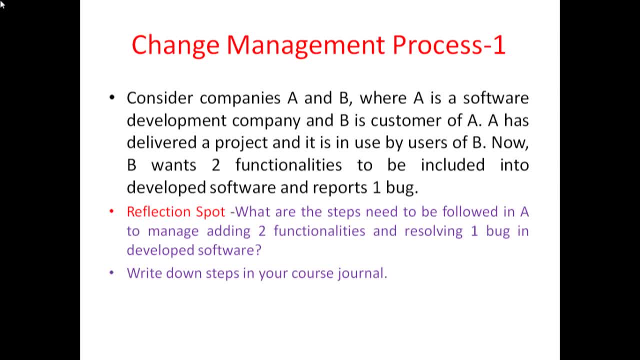 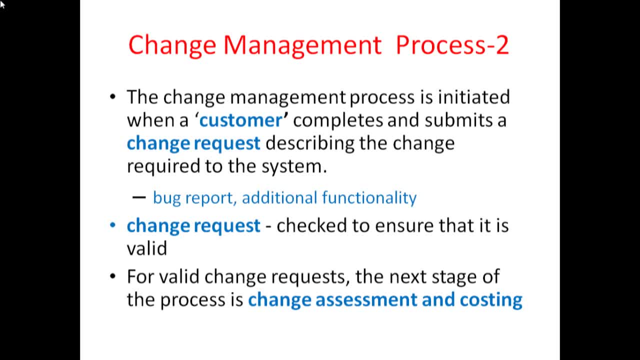 Answer this question and write in your course journal. What are the steps needed to be followed in A to manage adding two functionalities and resolving one bug in developed software and cost point of view, we will see the process. now you can see that there is a. 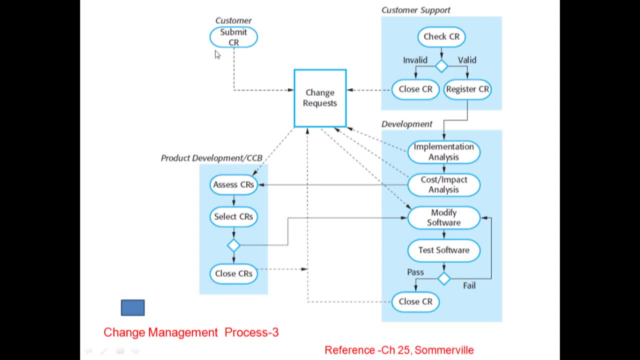 electronic form available which is submitted by the customer and a change request is submitted. so this change request could be electronic form and in that case this could be the database. there is a customer support team which first evaluates every arrived change request. it checks whether change request is valid or invalid. if it is invalid, then it needs to be closed with.